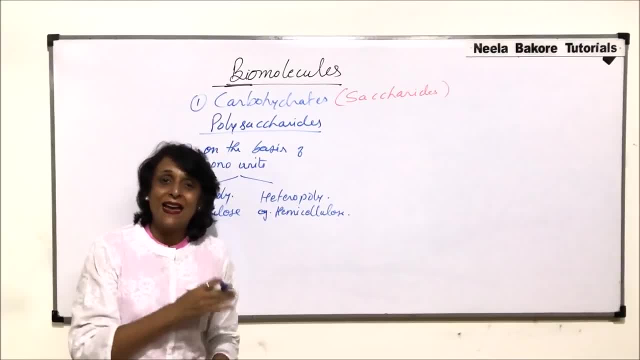 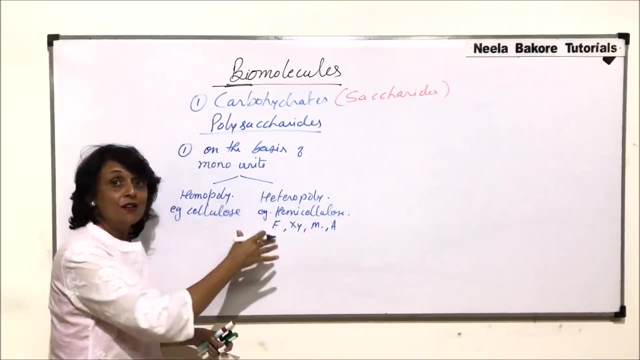 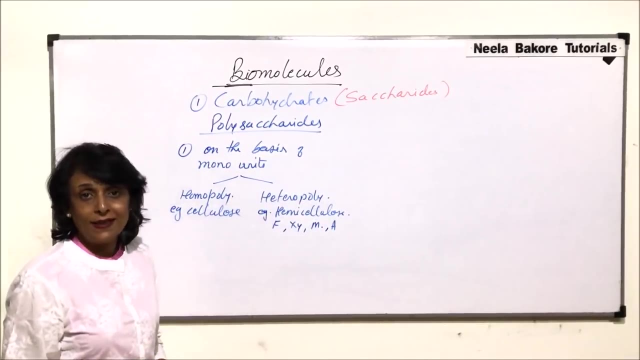 It is made up of galactose, mannose, xylose and albinose. So fructose, xylose, mannose and albinose. So there are different, different mono units which have combined to form the polysaccharide And that is why we call it heteropolysaccharide. This is one way of 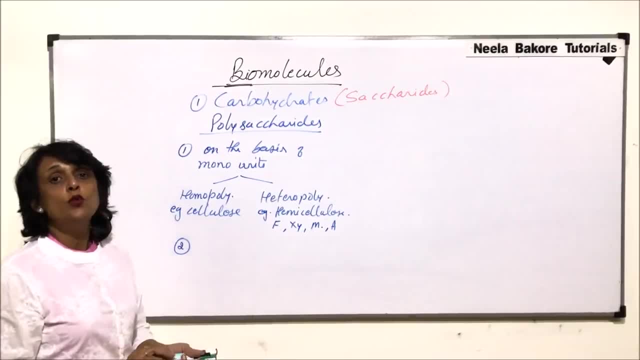 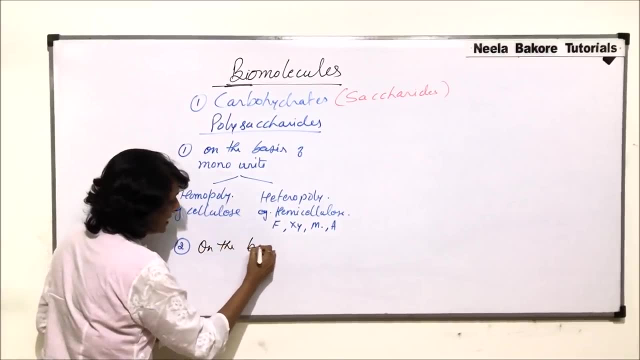 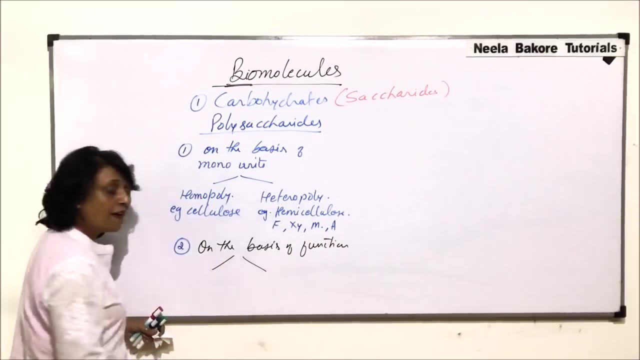 classifying them. The second is: what is the use, what is the function of these polysaccharides? So this is on the basis of the function or the role. Here also we can classify it into two categories: Storage polysaccharides. 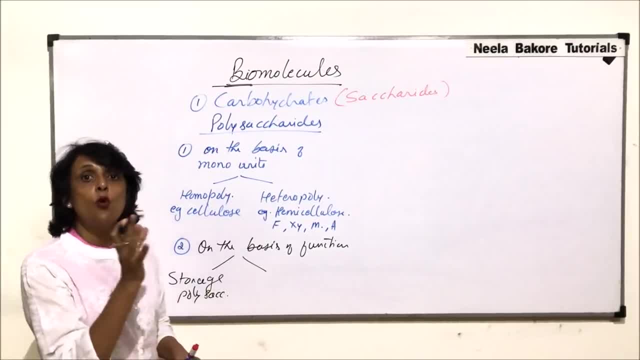 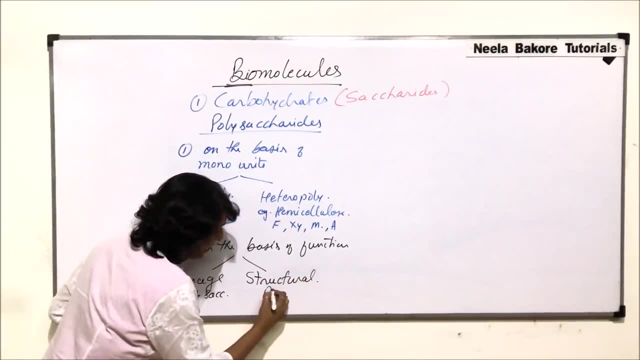 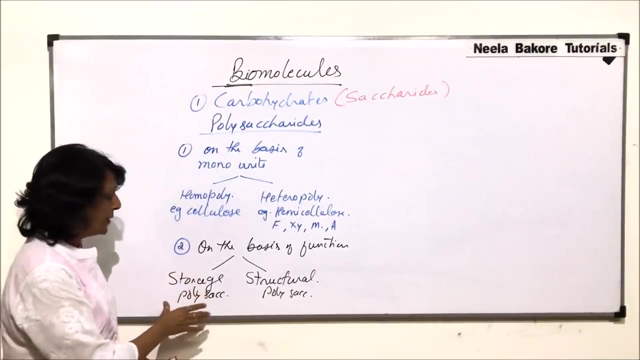 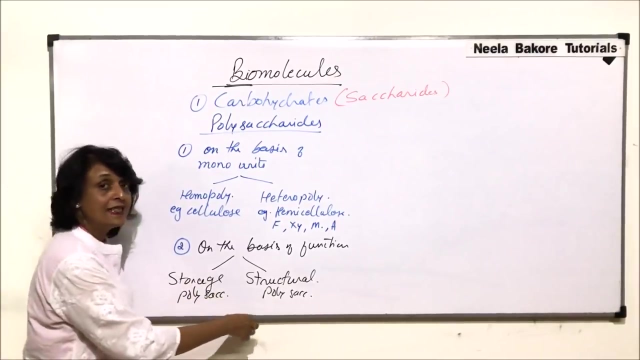 That means the polysaccharides which act as stored carbohydrate, And second is structural polysaccharides, which are performing a function of formation of a structure, For example starch. It is the stored carbohydrate, So it will come as storage polysaccharide And 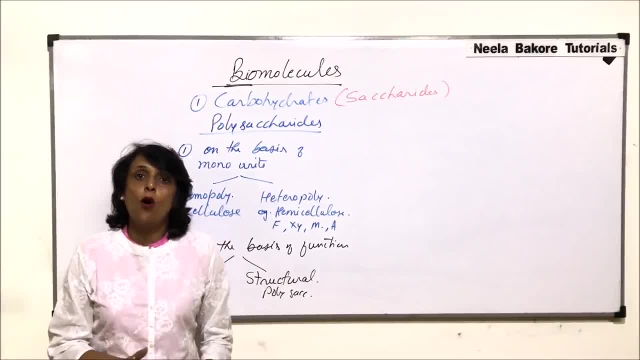 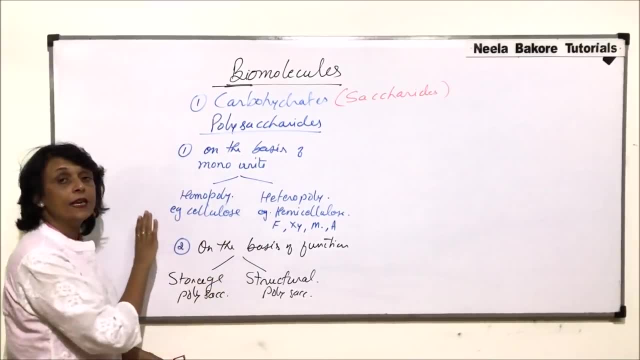 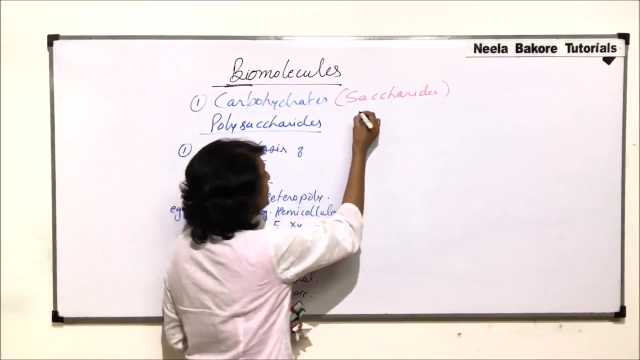 cellulose, which makes up the cell wall of plants, would become polysaccharide. So that is all the structure, polysaccharide. So these are the two ways in which we classify these polysaccharides. We will take up various polysaccharides, starting with starch. So first polysaccharide, that 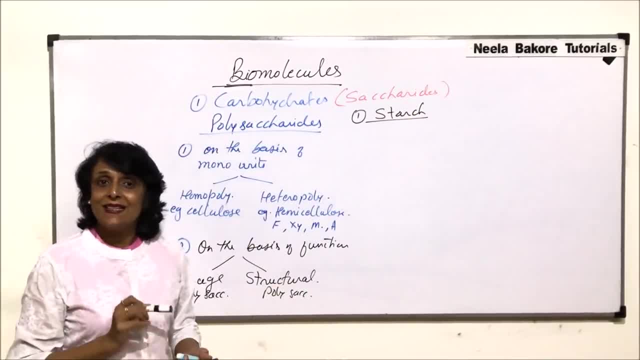 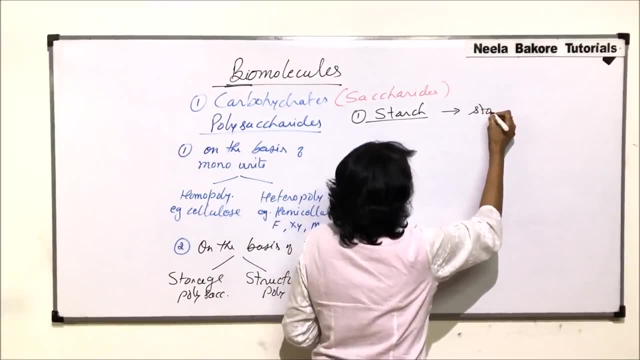 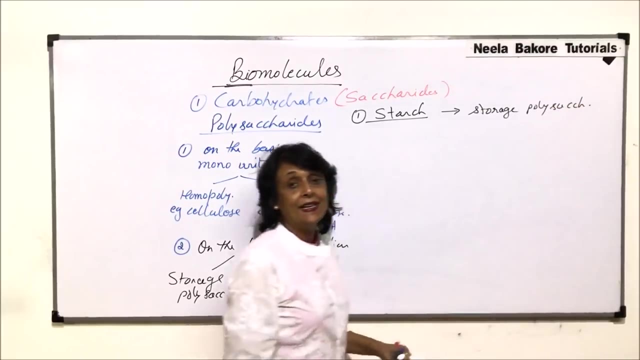 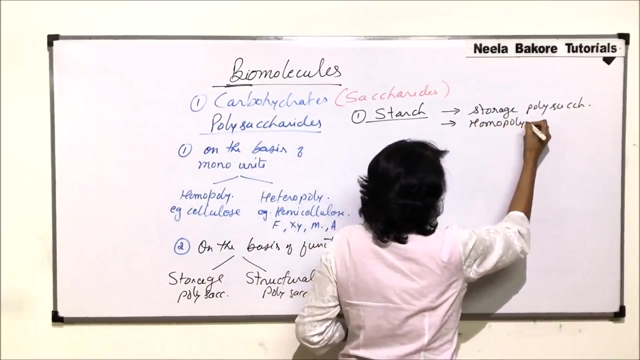 we are discussing is starch. It is the stored form of polysaccharide in plants. So it is storage polysaccharide, Starch And polysaccharide and it is a homopolysaccharide. It is again homopolysaccharide, That means it is made up of 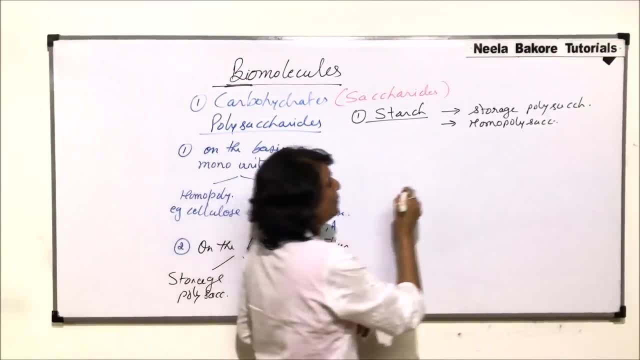 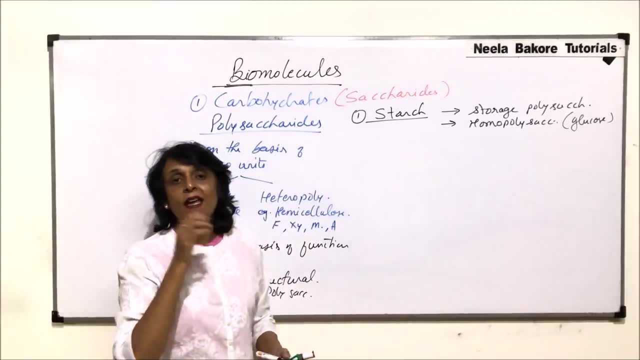 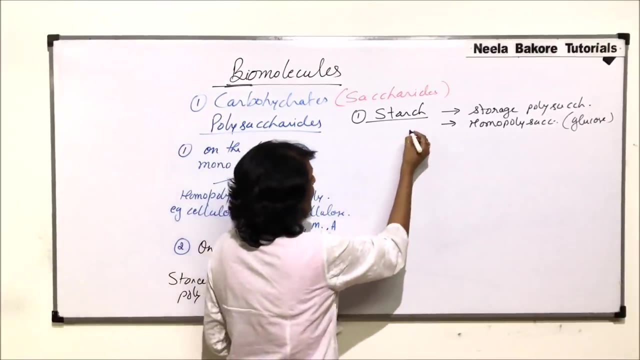 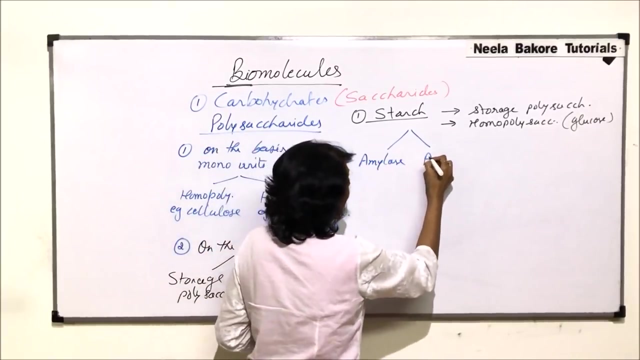 only one type of monounits. And what is that monounit? That monounit is glucose. So starch is made up of only glucose molecules. Now let us come to what the starch made up of. first, The starch is made up of two components. They are known as amylose and amylopectin. Both have glucose as their constituting substance. There are differences. In case of amylose, the number of glucose molecules are 200 to 2000.. In case of amylopectin, the glucose molecules are 2000 to 20000.. That means here the number of glucose molecules is more. The second thing: 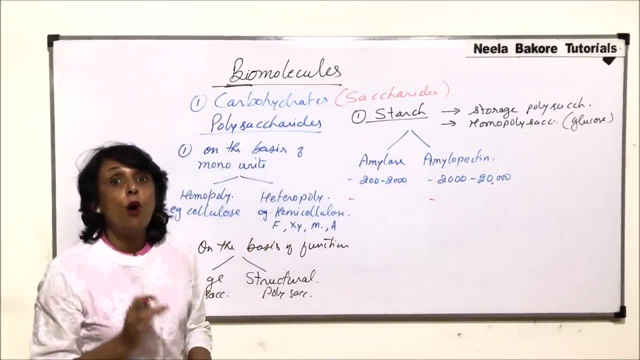 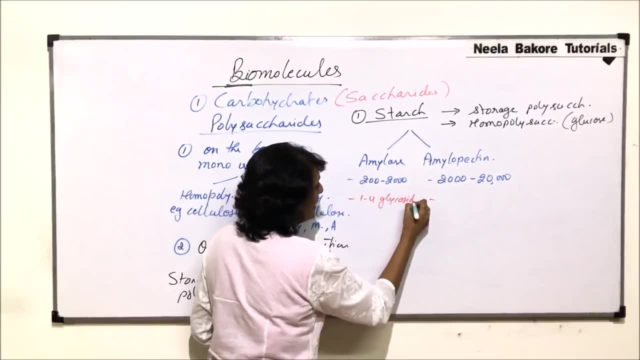 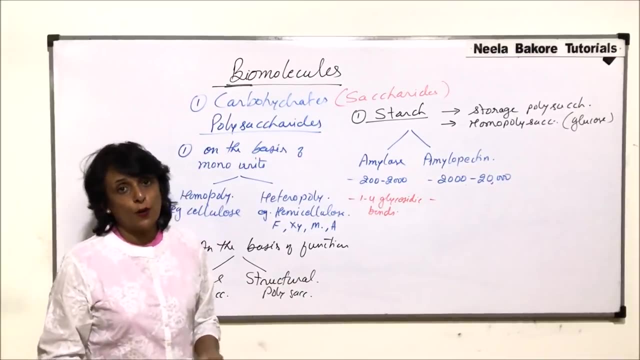 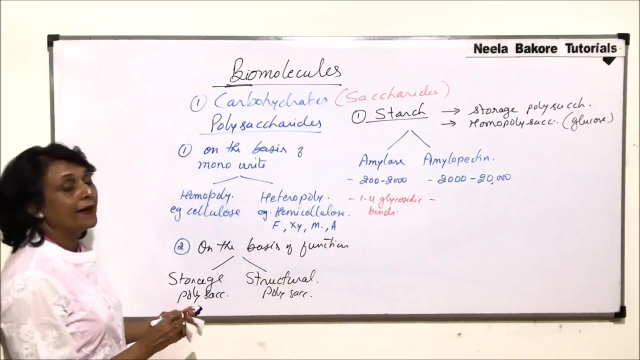 which is again very important is what type of bonds are present. Here. the bonds are 1,4-glycosidic bonds. Now, in the previous segments we talked about these bond formation, But we will quickly go over it because that is very essential in this part. If two glucose molecules join, 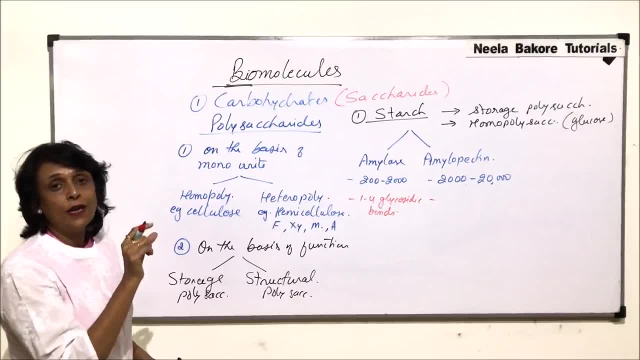 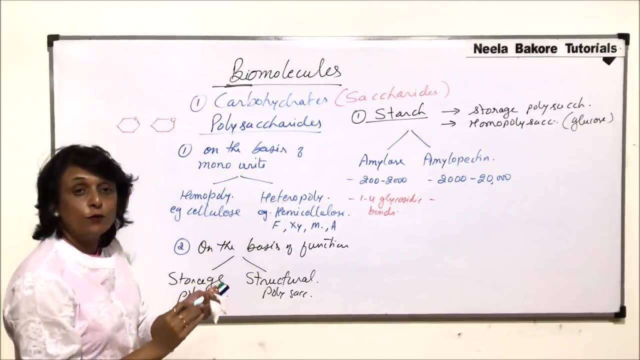 by this 1,4-glycosidic bond, then what kind of a structure is formed? Suppose we just make this small glucose molecule. Oxygen is here and it makes a bond with another glucose molecule Here, because it is a homopolysaccharide of glucose. we are talking only of glucose. This 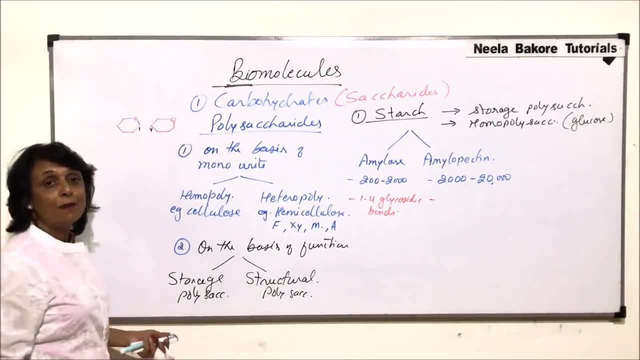 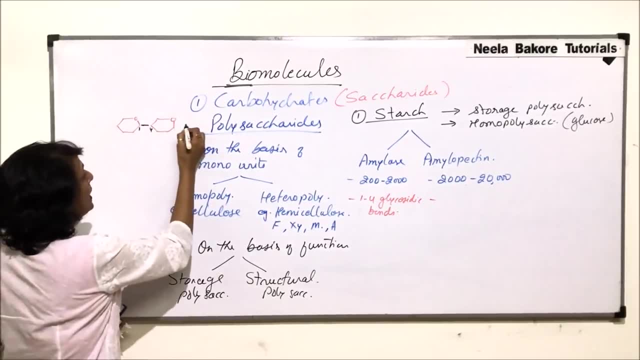 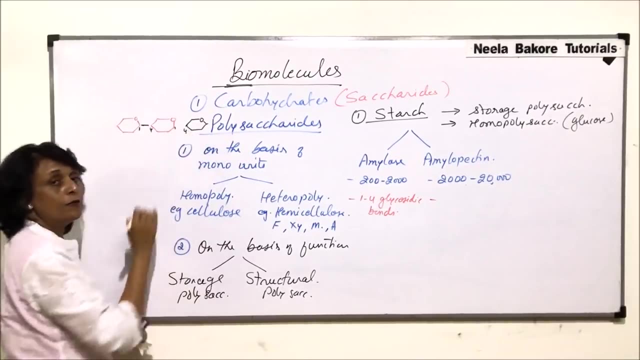 is carbon number 1 of this glucose and this is carbon number 4 of the other glucose. So the glycosidic bond which is formed is 1,4-glycosidic bond. If one more glucose molecule comes here again, it is going to be first carbon of this and fourth. So whenever we talk of 1,4-bonds, 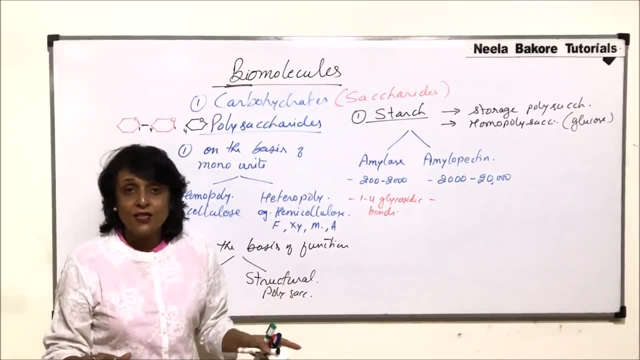 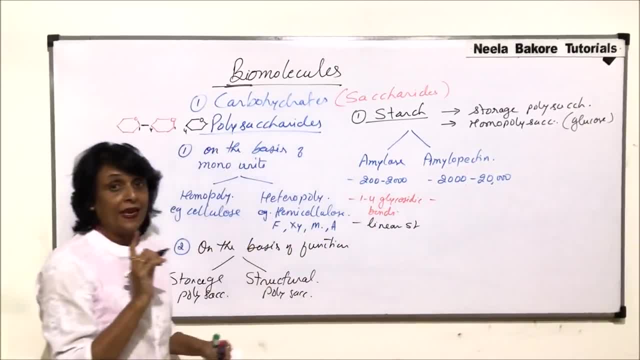 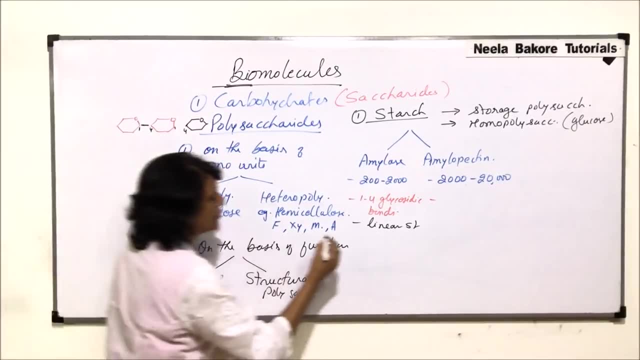 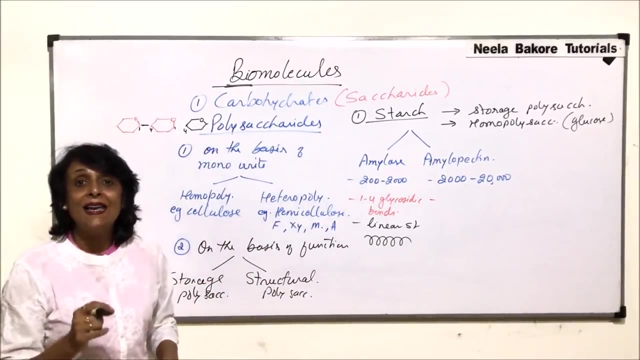 glycosidic bonds. it is a linear structure, but linear does not mean it has to be a straight line or a straight chain. It could be in this form also. So here the structure is like this: Though it is linear, no branching, but it is a highly coiled structure In case of amylopectin. 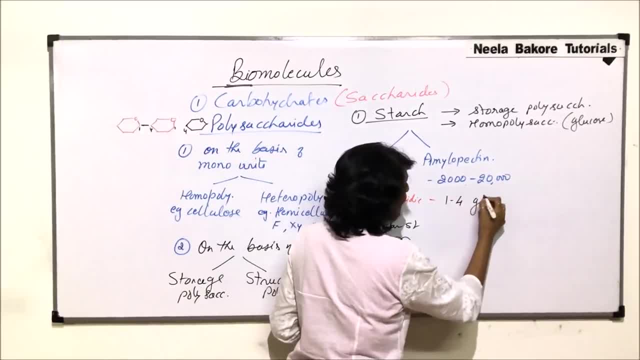 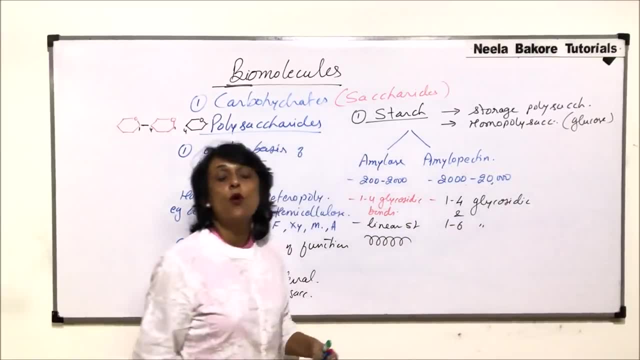 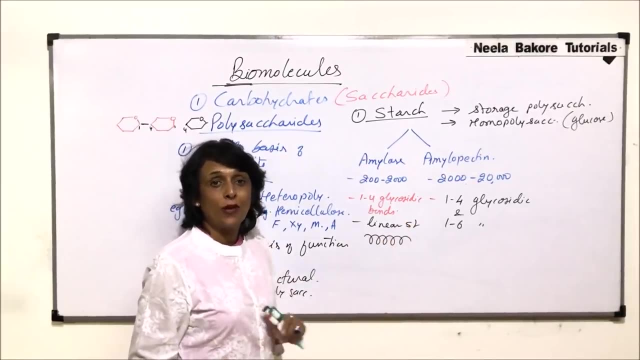 the bonds are 1,4-glycosidic bonds and there are one six glycosidic bonds also. so now let us see how the structure is due to presence of these two types of bonds. let me make this structure here. this is one glucose molecule. 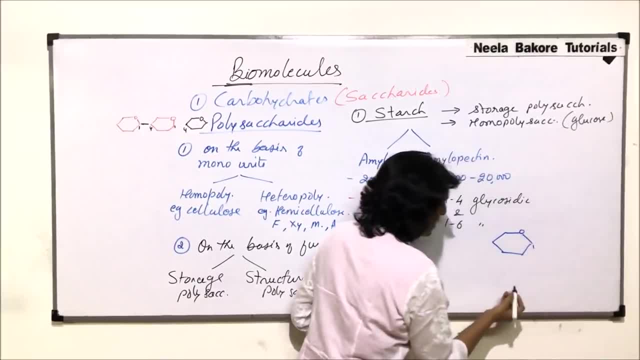 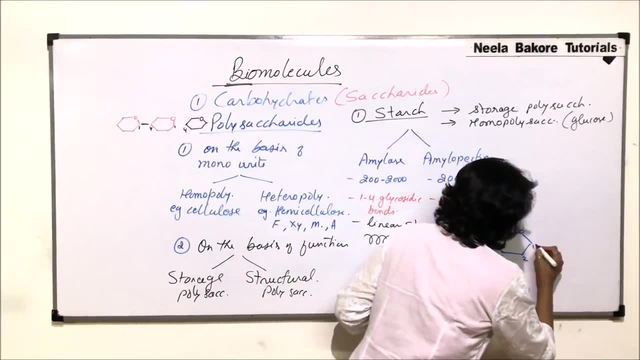 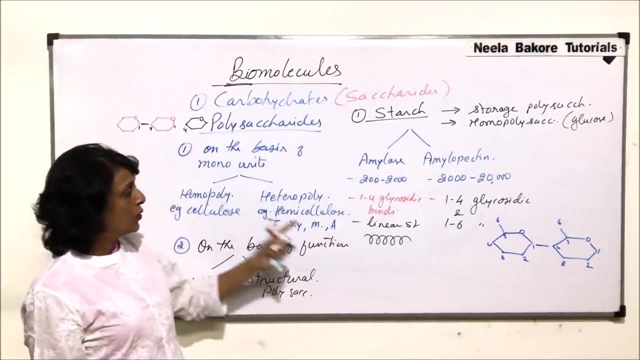 oxygen is here. this is carbon number one, two, three, four, five and six. if one more glucose joins in by glycosidic bond, this is another glucose oxygen, carbon number one, two, three, four, five and six. so, as we said in case of amylose, and we saw it here also, if it is only, 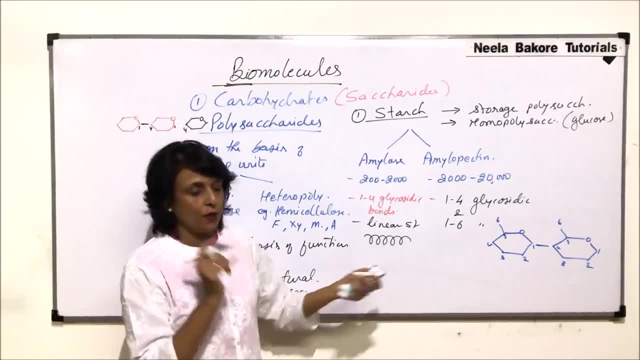 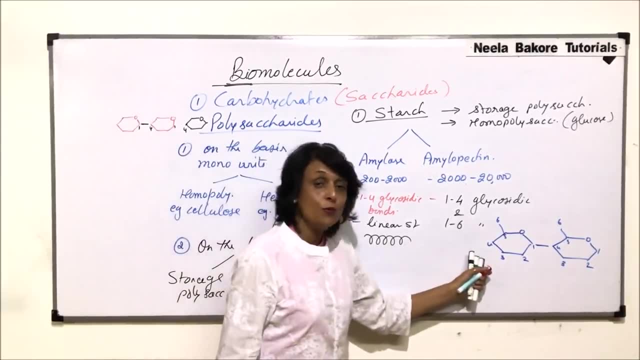 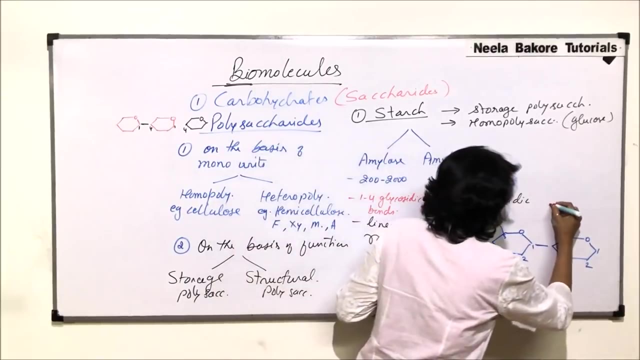 one four. it is going to be a straight molecule or a linear molecule. but if one six bond is formed, then there is branching. how is one six form? it is between the first carbon of one glucose and the sixth carbon of the other glucose. so if you make this glucose in this manner, 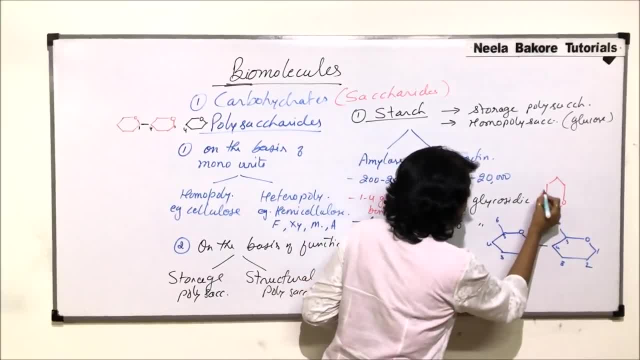 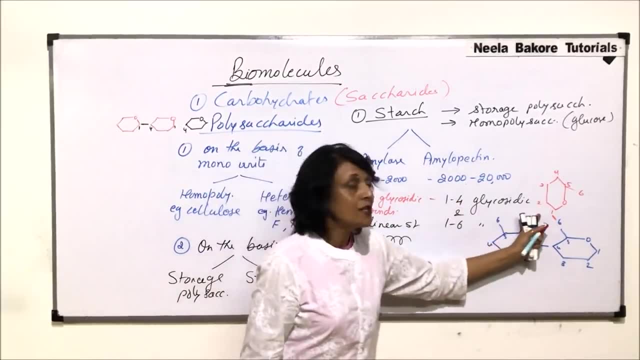 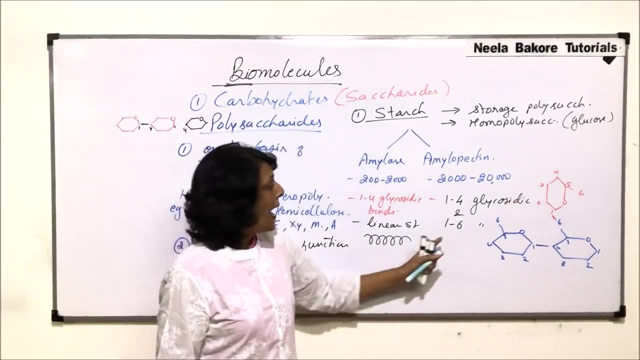 let us number the carbons. this is carbon number one, two, three, four, five and six, and the bond which is formed is between first carbon of this glucose and sixth carbon of this glucose. so the bond is one six glycosidic bond. as soon as one six is formed, we start seeing. 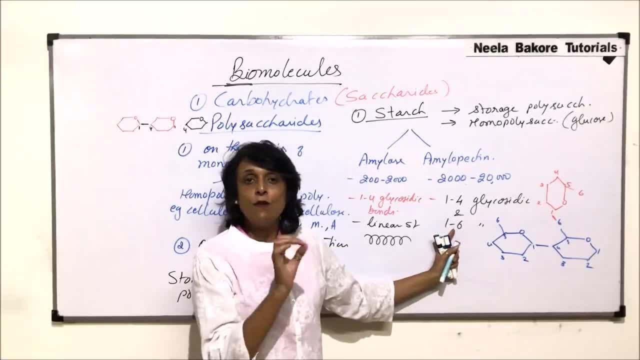 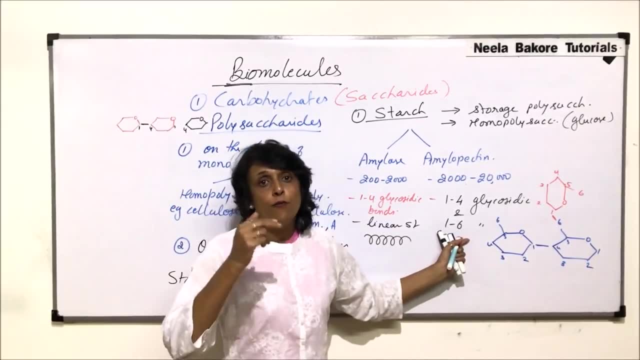 a branch. That means whenever we write 1,4-glycosidic bond, it tells us that it is only a linear molecule. And when we say it is 1,4 and 1,6, that means to that linear structure there is branching also. 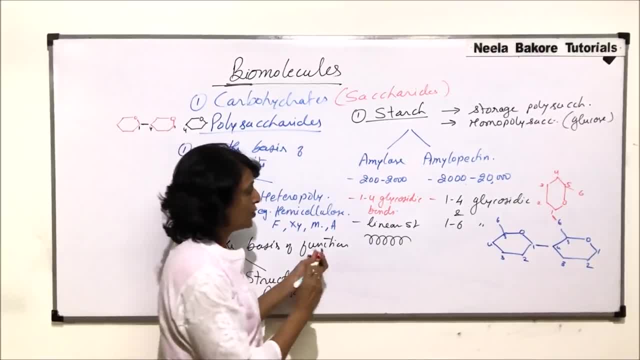 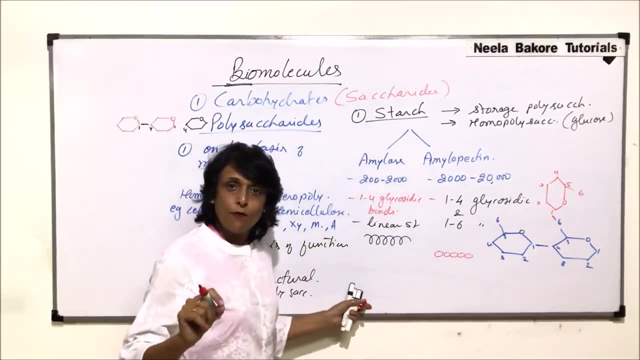 Here in case of amylose, we made it in the form of a coil structure. Here, in case of amylopectin, say, for example, these are the glucose molecules which are attached by 1,4 bonds When 1,6 are there. we would start seeing these kind of branching also. 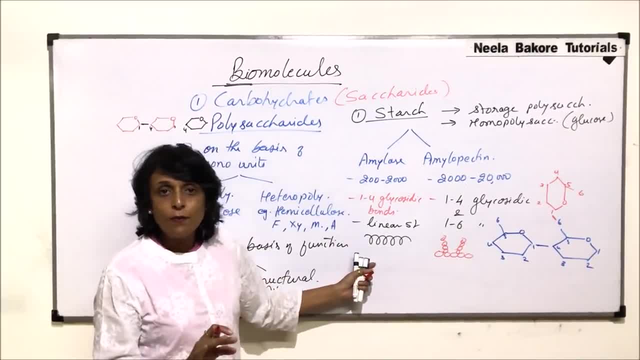 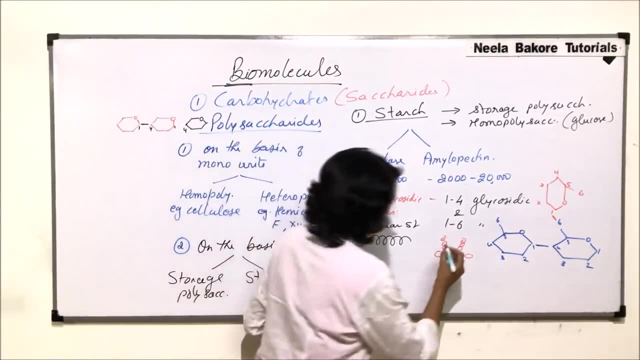 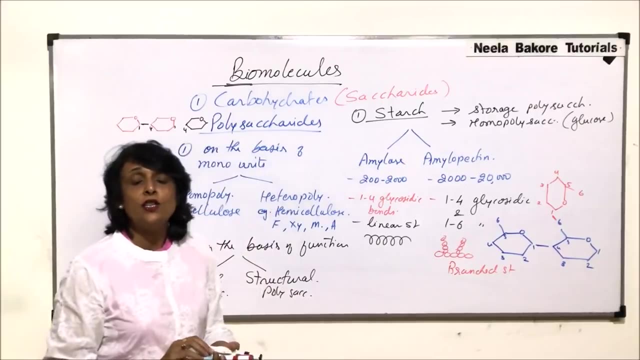 So amylose is a linear molecule without any branching. Amylopectin has 1,4,1,6- both, and that is why it is a branched structure. So this one is a branched structure. Ratio in which amylose and amylopectin are present in starch is: 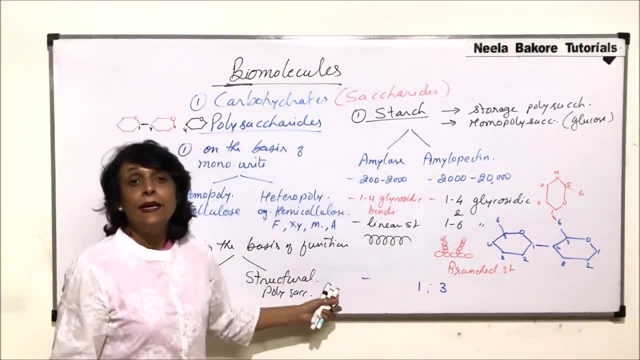 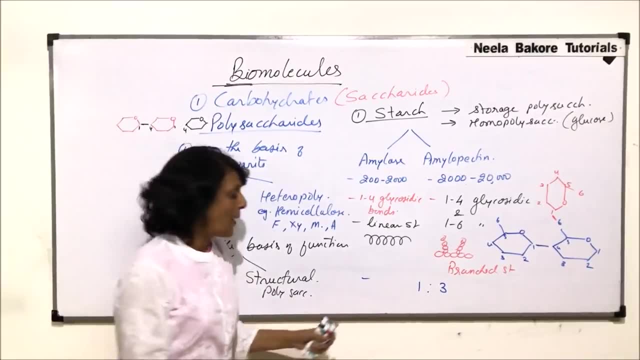 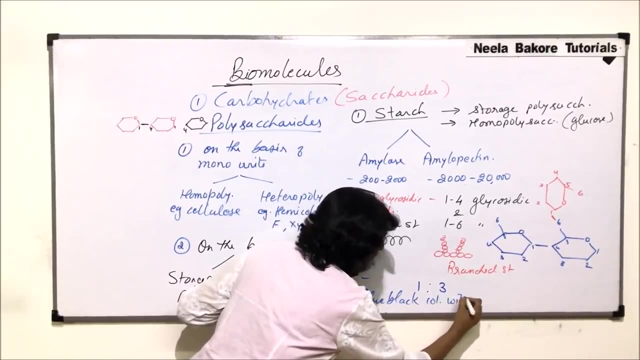 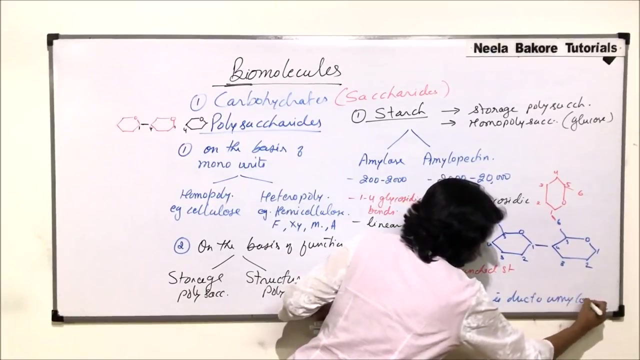 1 is 2.. 3. And the color- blue-black coloration of starch with iodine is due to amylose part. So blue-black coloration with iodine is due to amylose. That means this component of starch is responsible for this blue-black coloration. 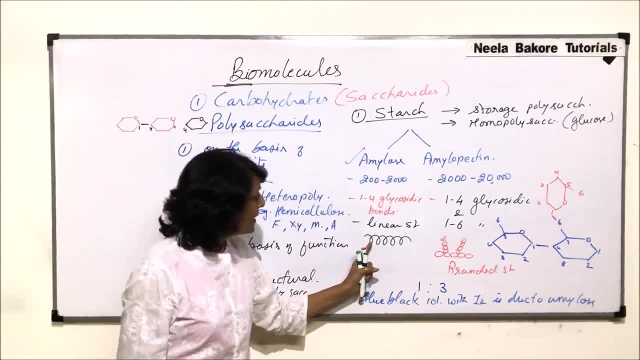 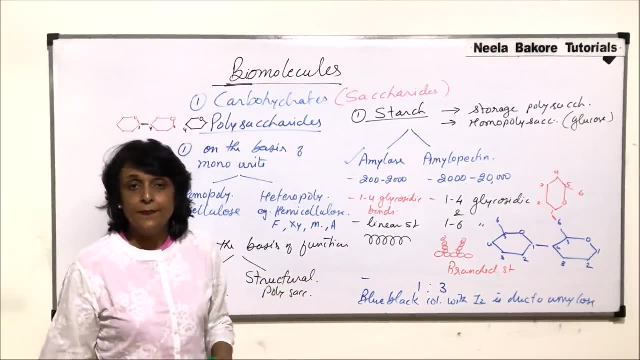 And the reason is iodine molecules. they get entangled into these coils which are formed in the structure. How is the starch present? The starch is stored. It is a storage polysaccharide. It is stored in various storage organs or structures. 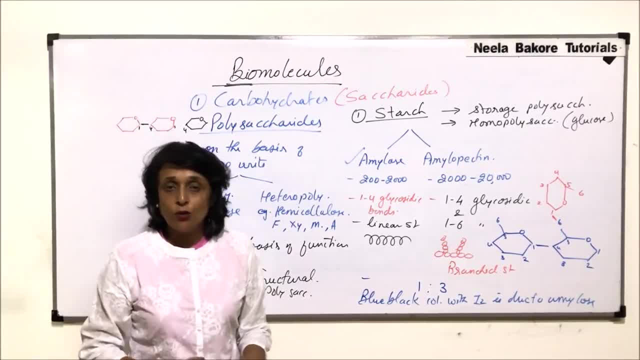 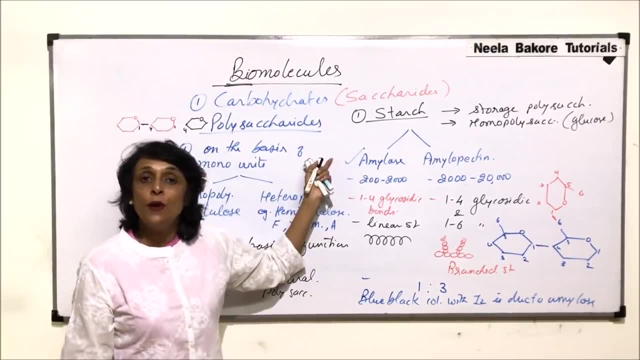 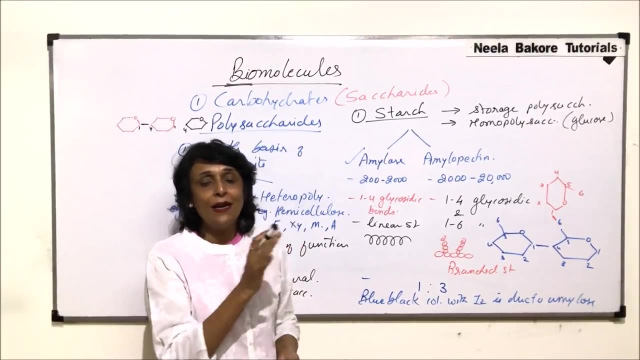 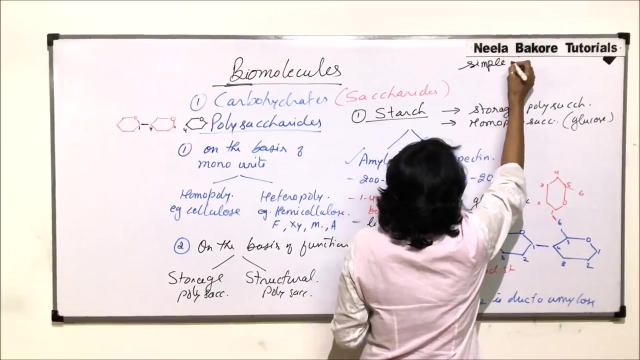 Those storage structures could be tubers, like in case of potatoes, It could be grain, as in case of rice, maize, etc. But the form in which starch is stored is known as a grain, and we classify these grains as simple grains or compound grains. what would be a simple grain, a simple grain? 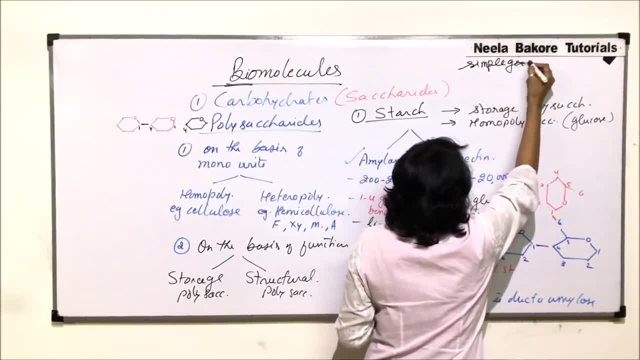 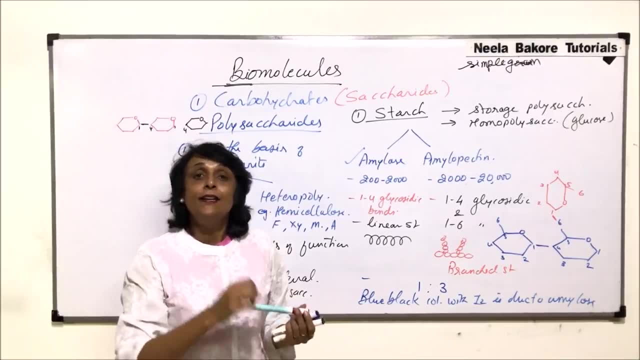 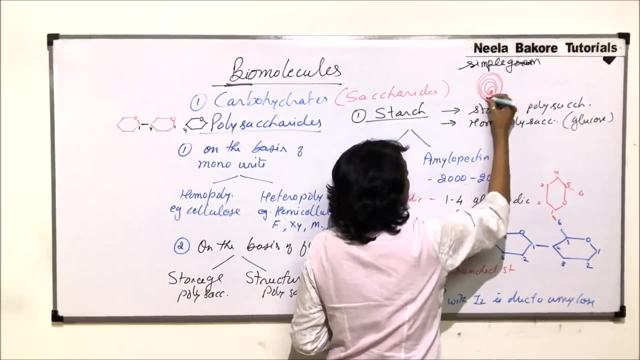 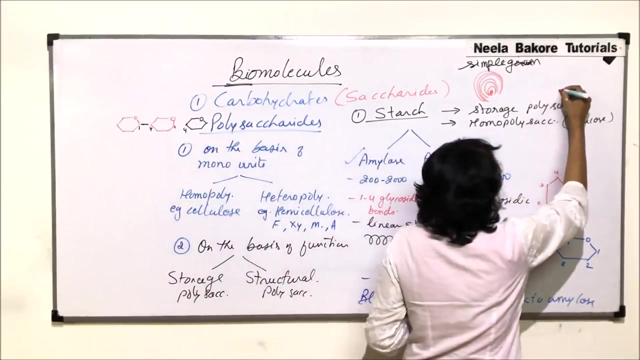 has simple grain has only one point around which the starch layers are deposited. that point is known as hylum and these layers are of starch. if there is only one hylum, then the grain is told as simple grain. but if there is, say this: hylum, few layers of starch, one more, hylum, few layers of starch, one more. 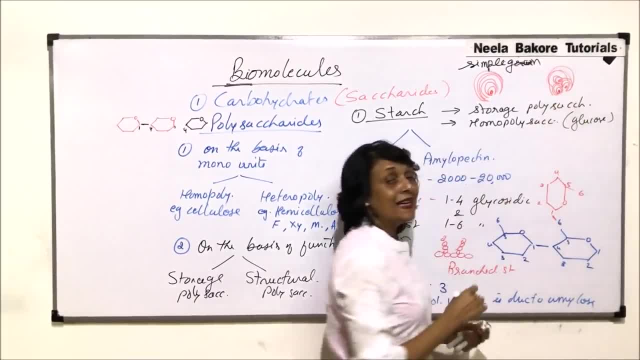 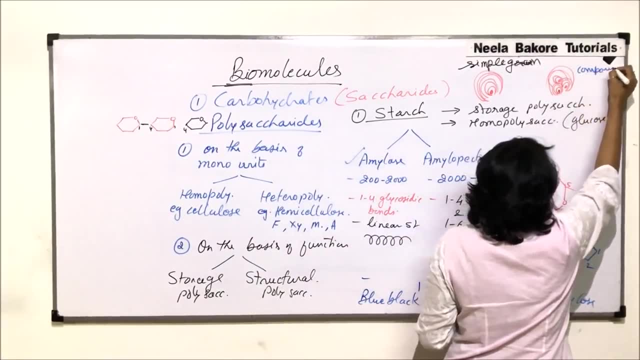 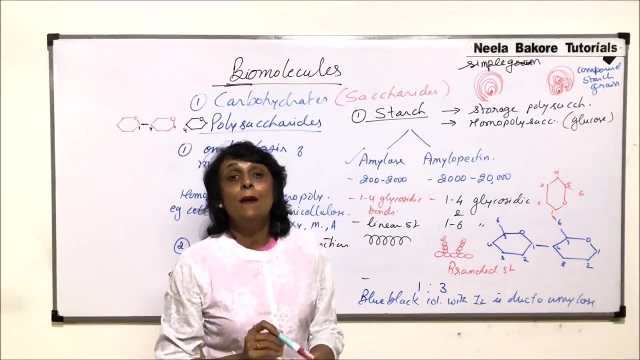 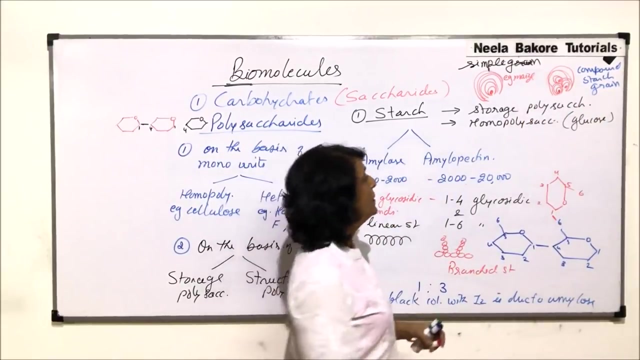 hylum and then there is a common sheath. then such type of starch grains would be termed as compound starch grains. so this is a compound starch grain. simple starch grain is found in maize, so here example is maize, whereas compound starch grain examples rice and potato. here we 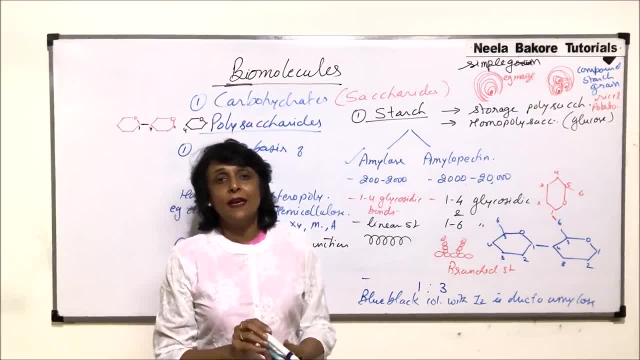 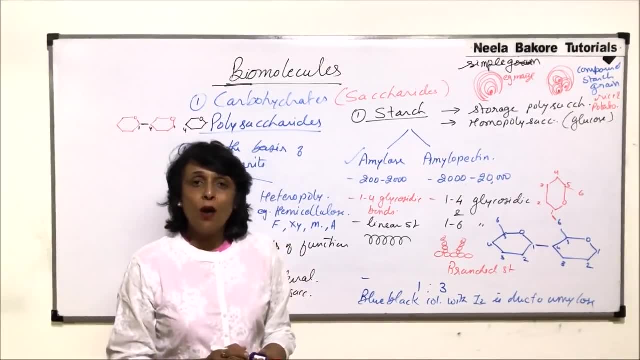 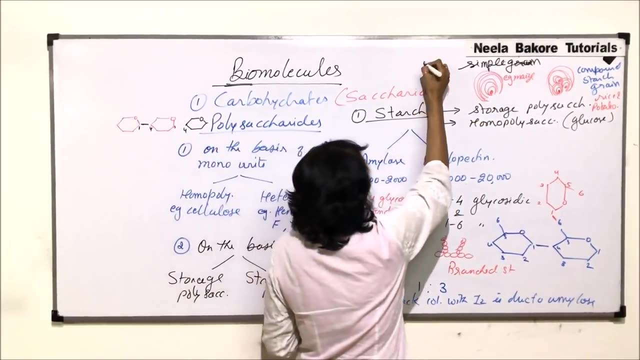 get these type of compound grains, simple grains. they can be of two types. depending upon the position of the hylum, they can be called as stay grain or rich grain. the other type of starch is known as the concentric or eccentric. the one that we have drawn here has hylum on one side, but if hylum is here, 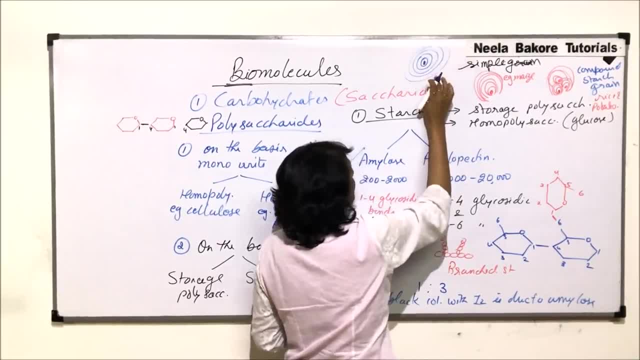 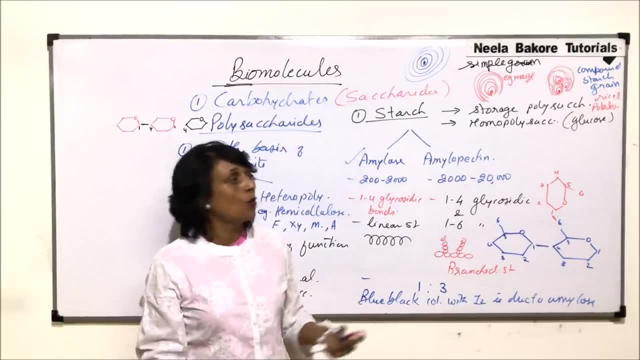 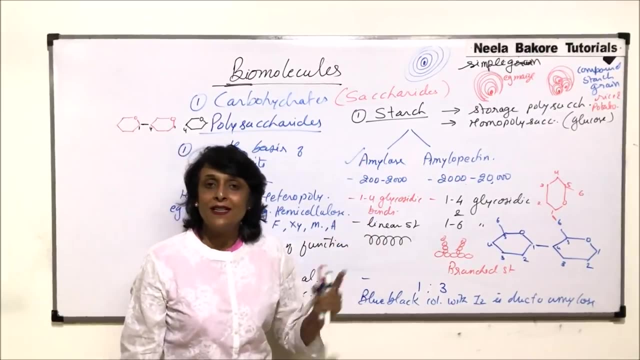 and the starch grains are surrounded like this, then it will be called a concentric, simple starch grain. so the grains, the starch which is stored, is in the form of grains and depending upon hylum numbers and position, we can classify them as simple or compound, or concentric or eccentric. 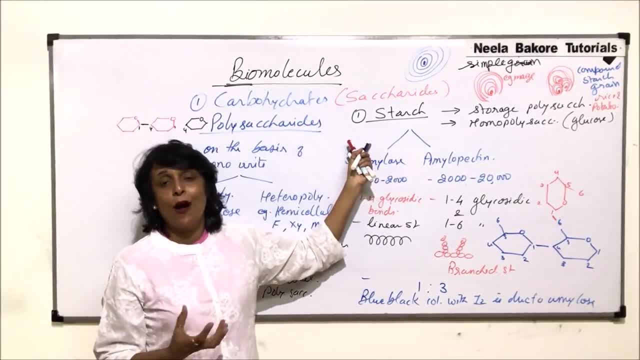 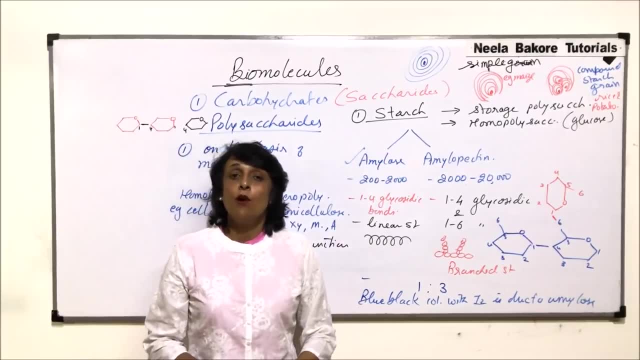 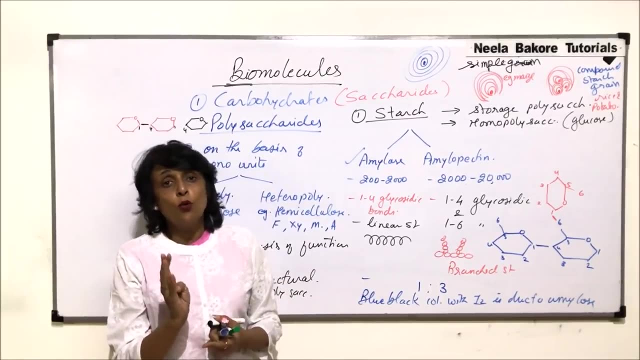 and this is the main carbohydrate which is stored. now, as we are talking of starch, which is a storage polysaccharide, we also need to understand one very simple thing: plants synthesize carbohydrates as glucose. this glucose is a reducing sugar highly reactive, so when it is transported, it 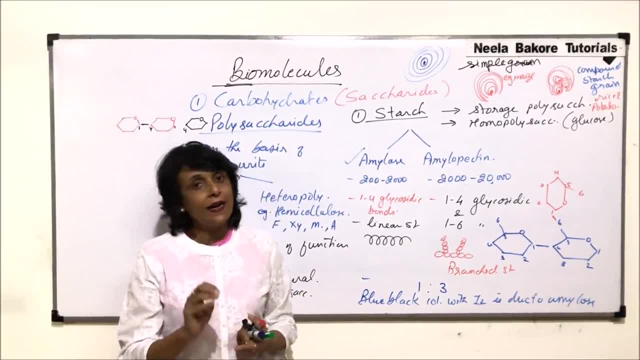 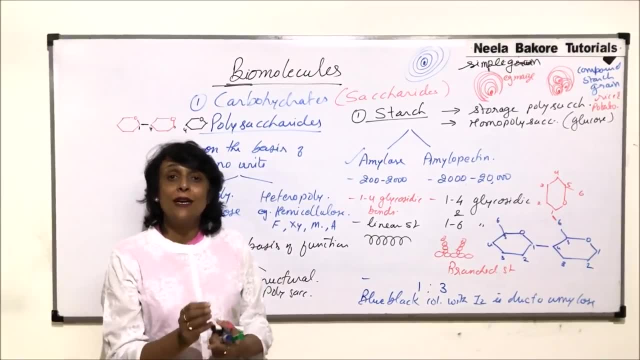 is converted to glucose. so when it is transported, it is converted to glucose. so when it is transported into sucrose, sucrose is a disaccharide non-reducing sugar, so it is not going to react with anything. so synthesized as glucose, transported as sucrose and stored as starch and when the plant wants to. 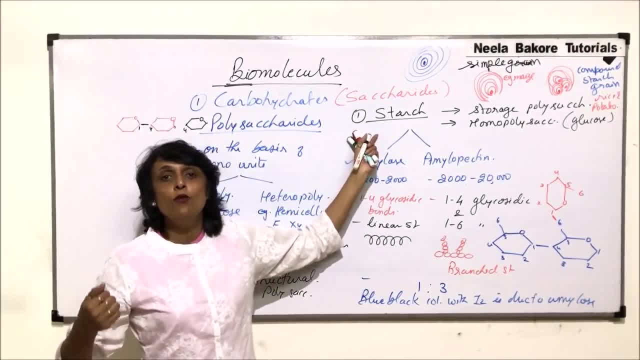 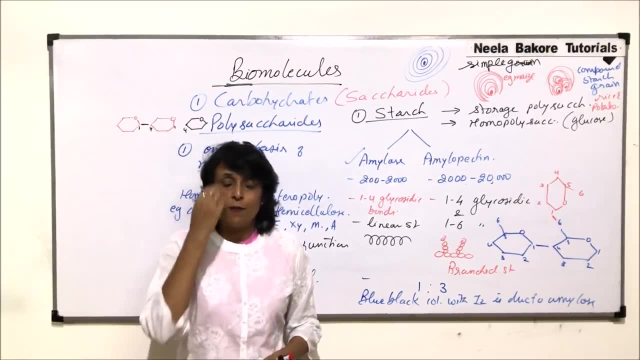 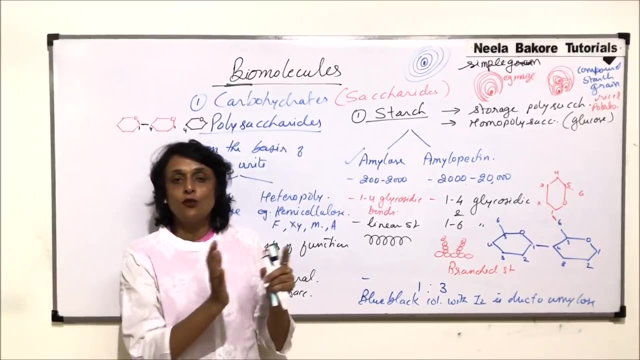 use it. this starch will be ultimately broken down into glucose and then it will be used. so why not store glucose itself? because ultimately the plant has to use glucose. one reason is glucose is highly reactive. it is a reducing sugar, so it has to be converted into a non-reactive substance. 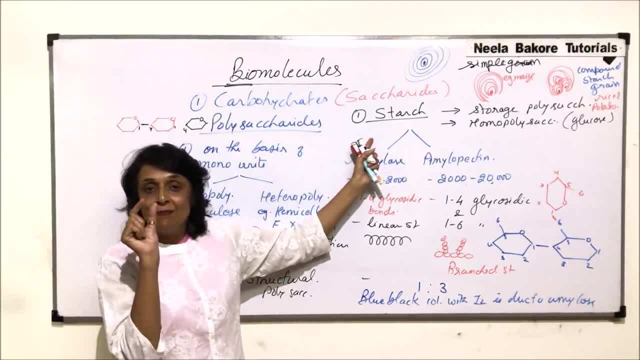 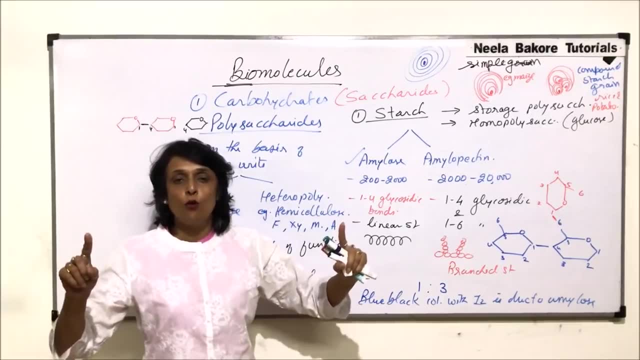 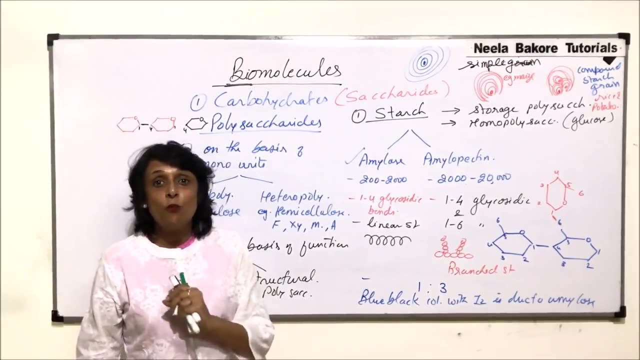 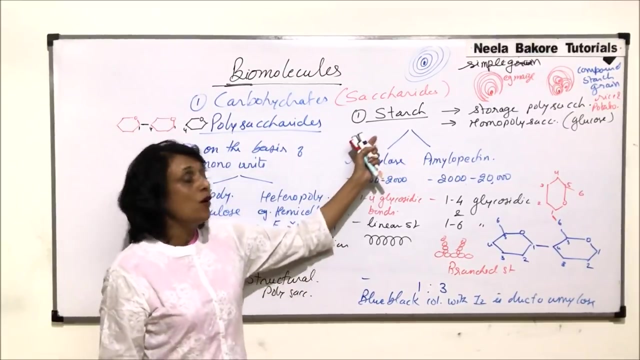 secondly, every time a bond, glycoside bond, is formed, one water molecule is eliminated. so if hundred glucose molecules are joining together, then how many water molecules would be removed? 99 water molecules would be removed. that means those many hydrogen and oxygen atoms less. that means those many hydrogen and oxygen atoms less. 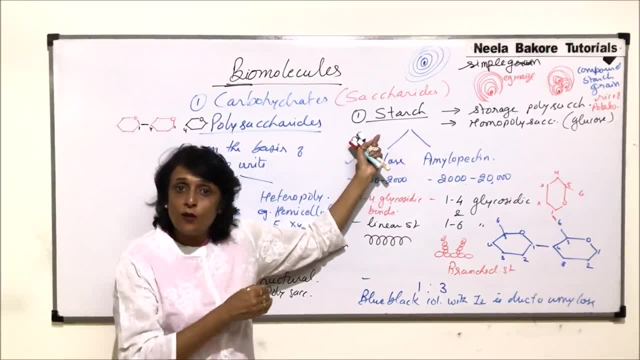 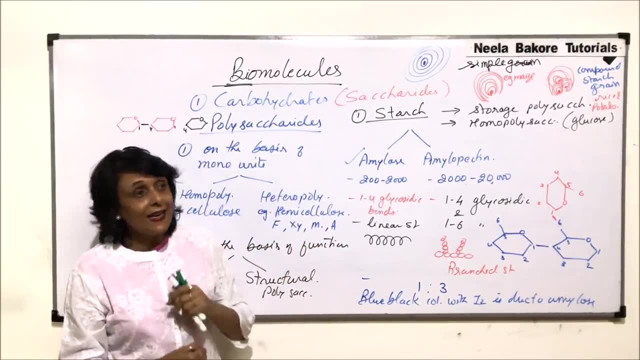 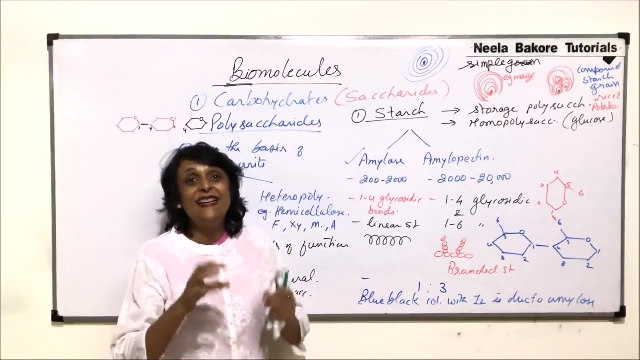 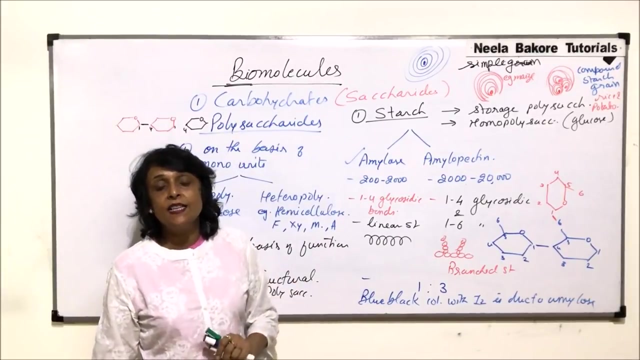 sill. Sirin, a polysaccharide, is an easier option because it gets compact and to store of contact molecule is always going to be an easier option. secondly, how do we break this much? by formation of this bar, water was lost. it is fine dehydration synthesis to break this bond. water has to be added. and that is not all digestive enzymes. 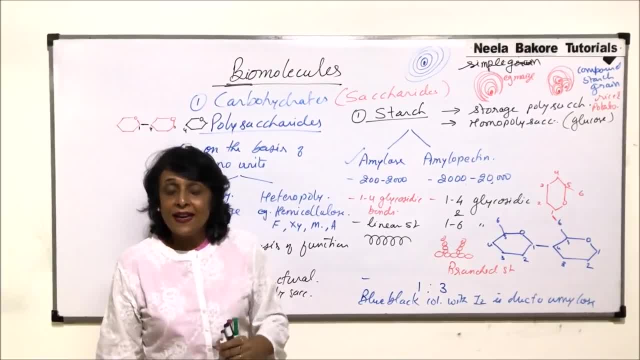 hydrolyticOLL cake enzymes. they layer, fertilize, then avoid the lack of hydrogen. so wrapped up as glucose and glucose they are gone to given the arable reviewm deutlich bacteria in order to have it didn't lose jagme belts as� break the bonds by addition of water, So breaking the polysaccharide to release monosaccharide is. 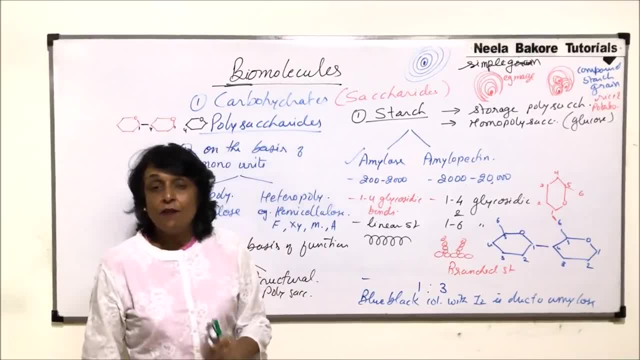 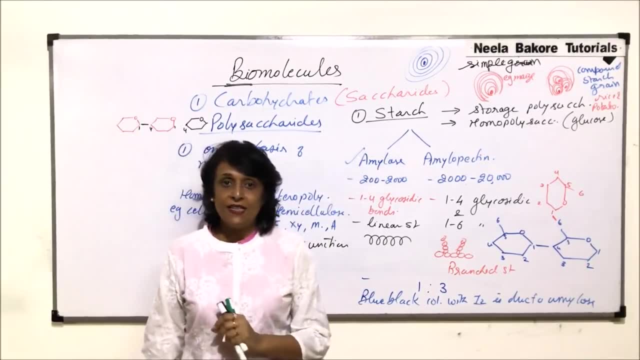 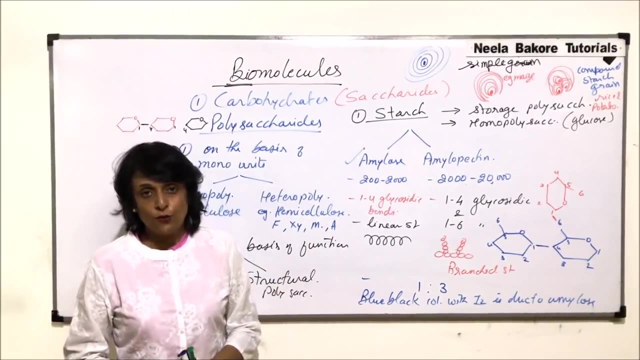 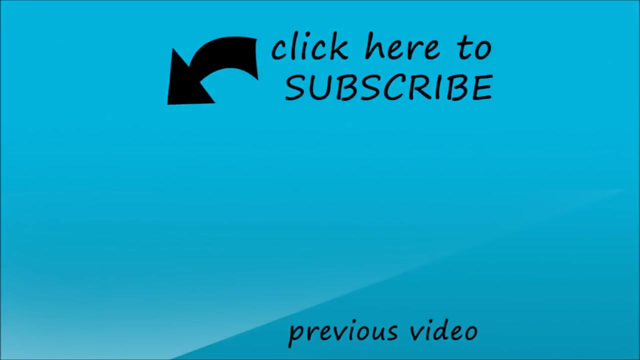 not a very difficult task. It can be easily achieved. But storing is an important thing, and that is why carbohydrates are stored as polysaccharides. After starch we will take up the next polysaccharide, that is, cellulose. Thank you for watching. 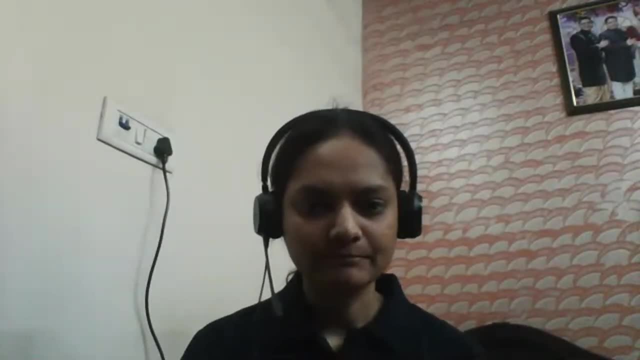 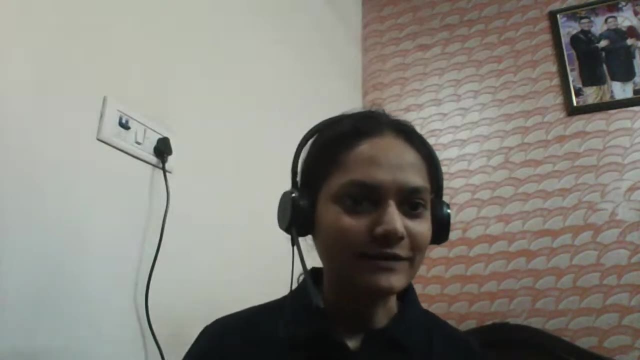 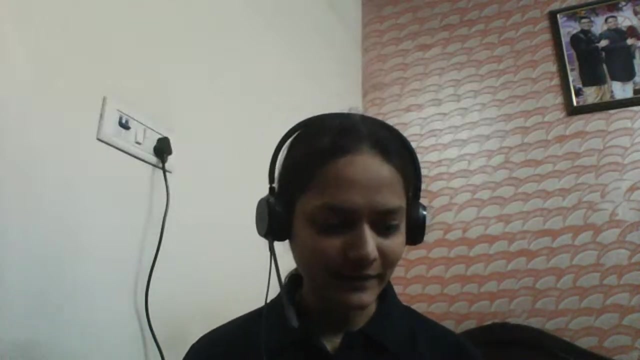 Hello everyone, And we are back for another Python session And let's wait for a couple of minutes for more people to join in, And it's good to see you all here again. So this is one of the last Python sessions we are having in the current series that we concluded. 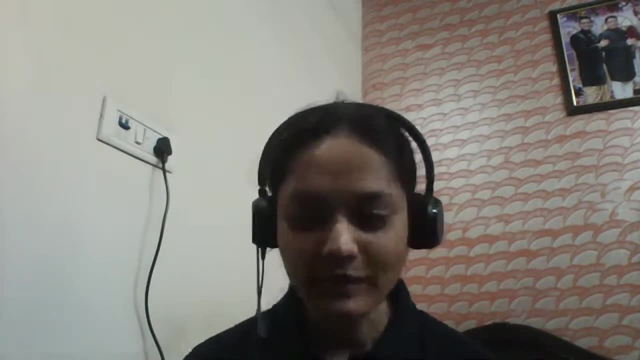 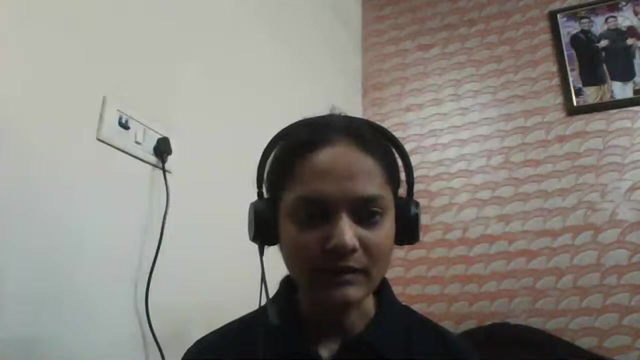 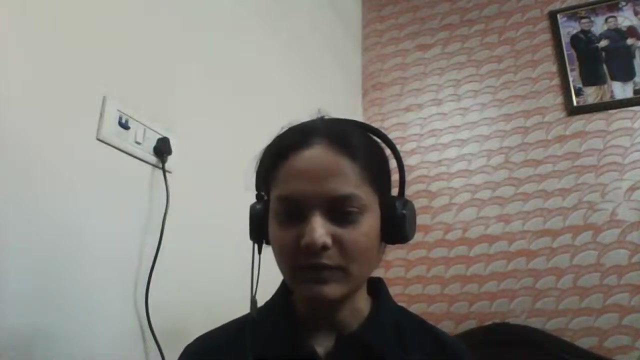 So, yeah, today we are going to be covering a Python case study And I hope you are all excited about it. So before that we'll discuss a bit more And also like what all we went through, Just a quick revision of our all eight sessions And also a little bit about 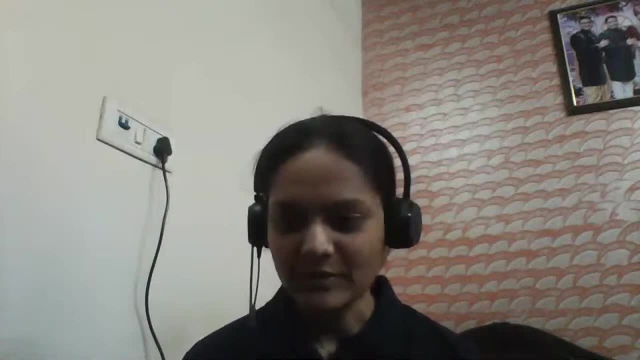 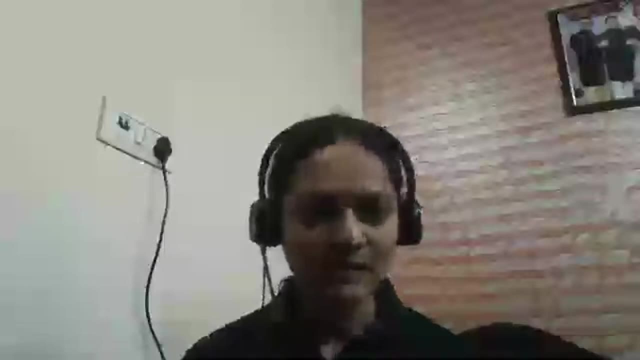 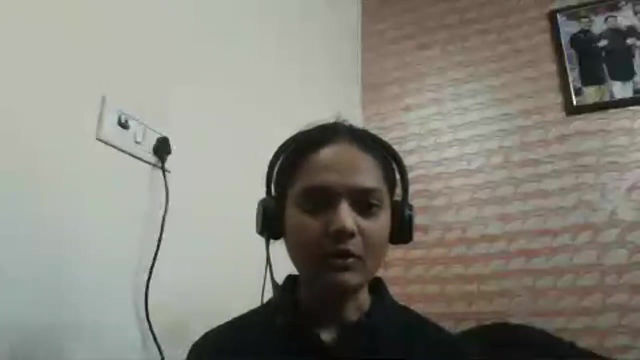 our company. So let me just kick off And I'll start with an introduction for Infinii Data Academy. So, Infinii Data Academy: we are a Python and Data Science training group And we provide bespoke trainings to all the people who are looking to upskill themselves in the field. 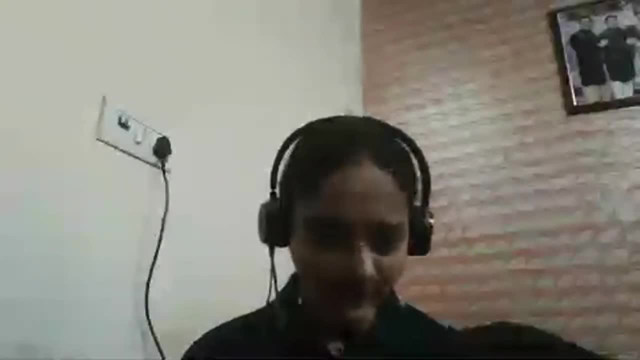 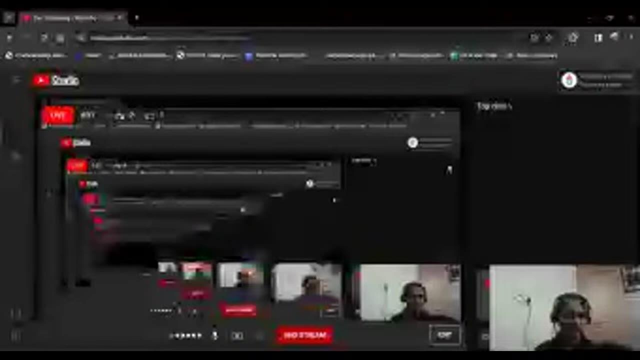 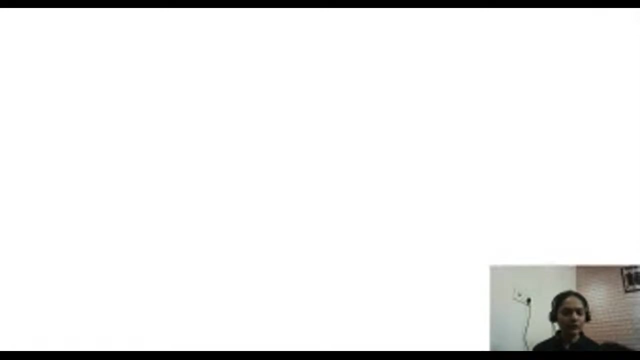 of data science and analytics And I'm just going to share my screen and show you a little bit about the Infinii Data Academy, Like what about their presence and our pages? So you can follow us on the LinkedIn and YouTube, And we are active on all social media. 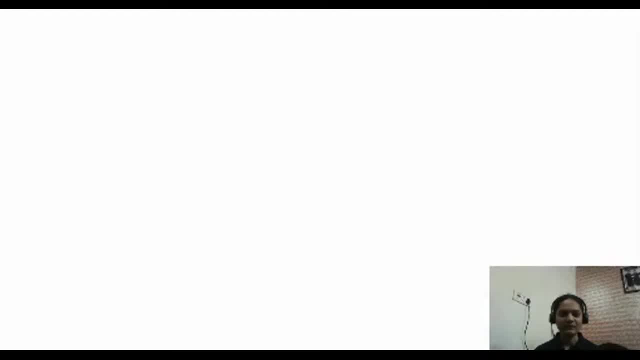